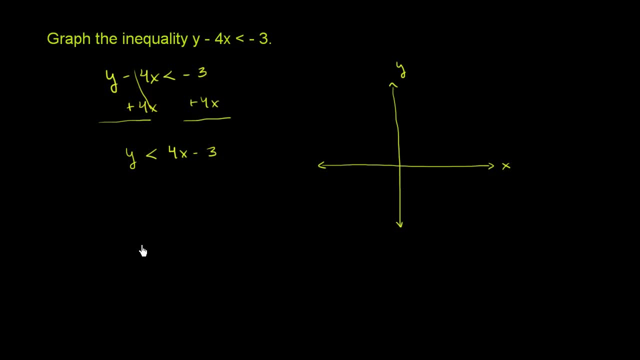 will be all of the area below that, all the y values, less than that. So let's try to do it. So the boundary line would look like this, So let me write it over here. So we have a boundary at y is equal to 4x minus 3.. 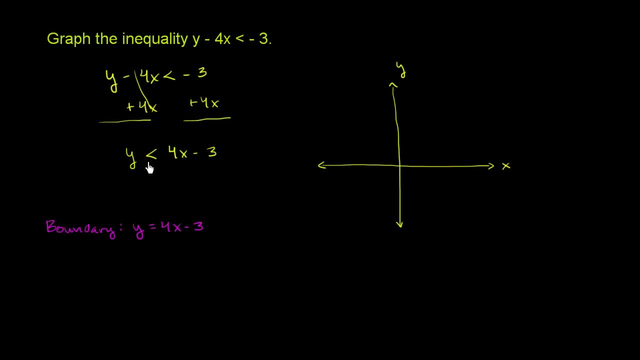 Notice, this isn't part of the solution. This isn't less than or equal, It's just less than. But this will at least help us draw essentially the boundary. So we could do it two ways, If you know: slope and y-intercept. 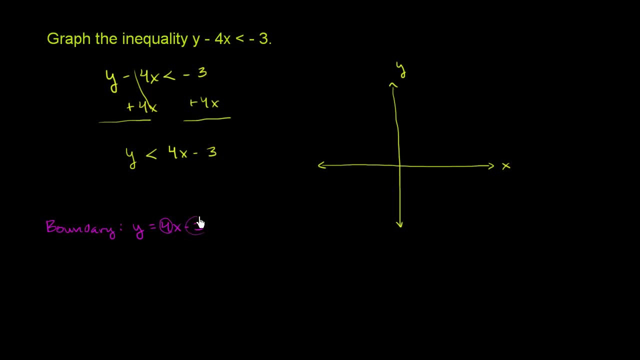 you know that 4 is our slope and that negative 3 is our y-intercept. Or you can literally just take two points and that'll help you define a line here. So you could say: well, when x, You could say when x is equal to 0, what is y? 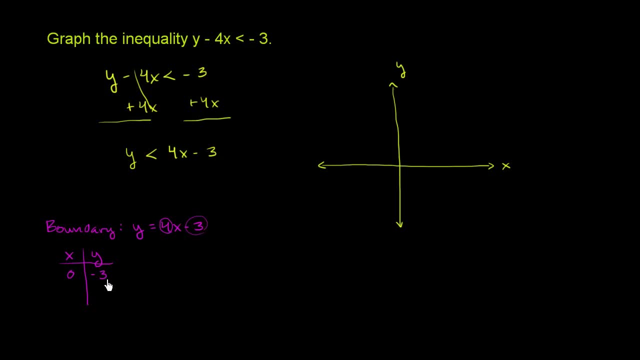 You get 4 times 0 minus 3.. You get y is equal to negative 3. And we knew that because it was the y-intercept. So you have 0, and then you have 1,, 2,, 0, and negative 3.. 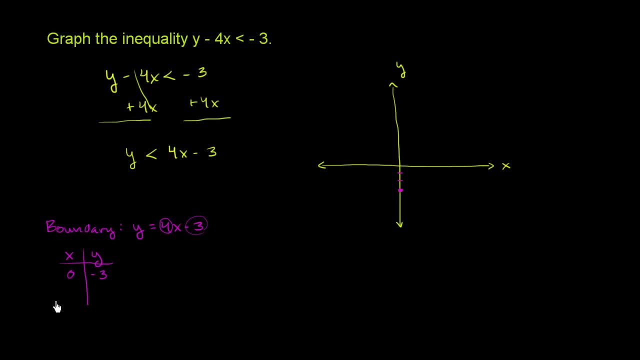 And then you have the point, And then you have the point. Let's say: when x is equal to, I don't know. let's say when x is equal to 2.. When x is equal to 2, what is y? 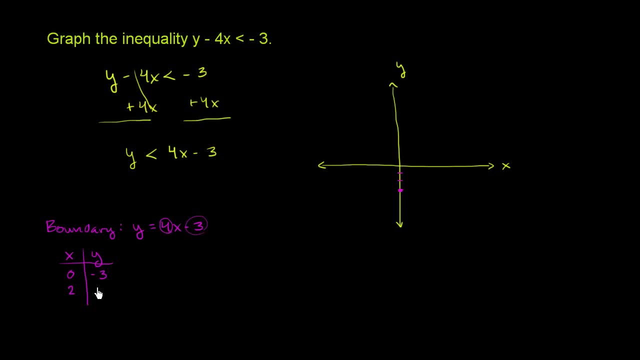 We have: 4 times 2 is 8 minus 3.. y is then going to be equal to 5.. So you go 1, 2, and you go 1,, 2,, 3,, 4,, 5.. 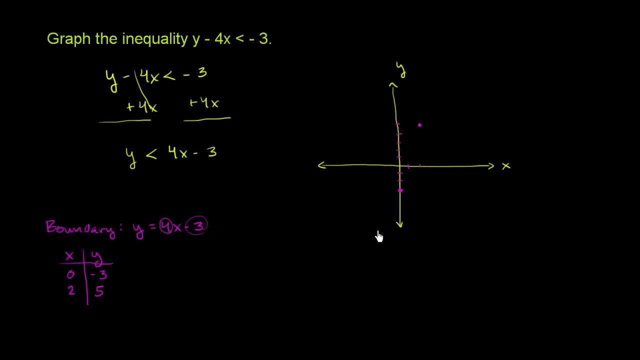 So you have that point there as well, And then we can just connect the dots. Or you could say: look, there's a slope of 4.. So every time we move over 1, every time we move 1 in the x-direction, we move up 4 in the y-direction. 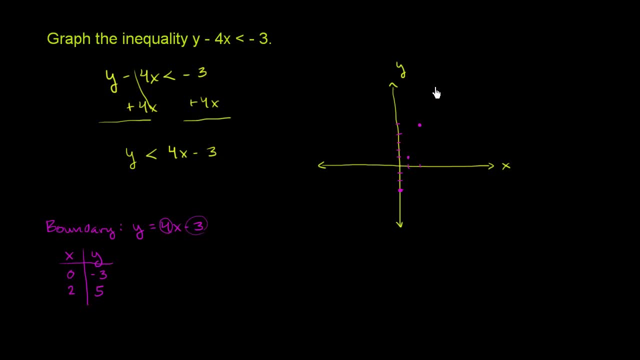 So you could draw it like that. So the line will look something like this And I'm just going to draw it. I'm going to draw it at a dotted line Because, remember, this isn't part of the solution. Actually, let me draw it a little bit neater. 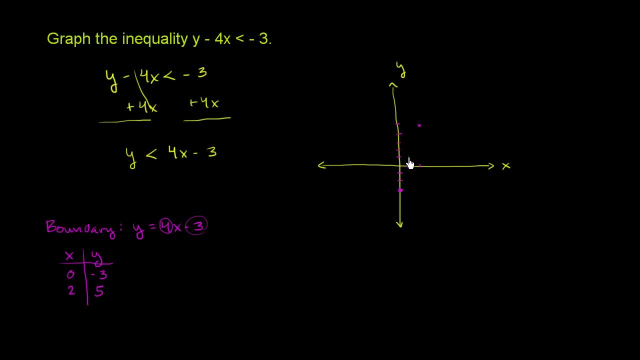 Because that point should be right about there, This point should be right about there. And then this boundary line I'm going to draw as a dotted line, So it's going to look like it's going to look something like that, And I draw it at a dotted line to show that it's not part of the solution. 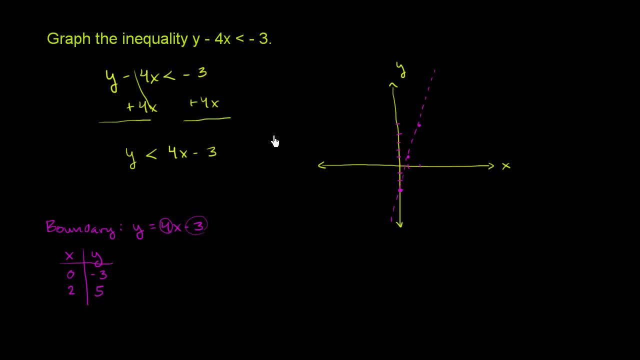 Our solution is the y's less than that. So for any x. so you pick an x here. If you took 4x minus 3, you're going to end up on the line, But we don't want the y's that are equal to that line. 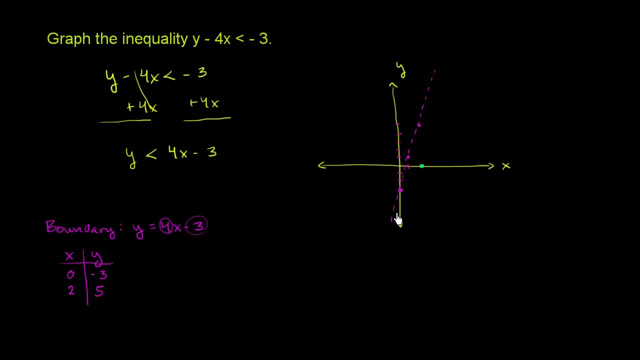 We want for that particular x, the y's that are less than the line. So it's going to be all of this area over here. We're less than the line and we're not including the line, And that's why I put a dotted line here. 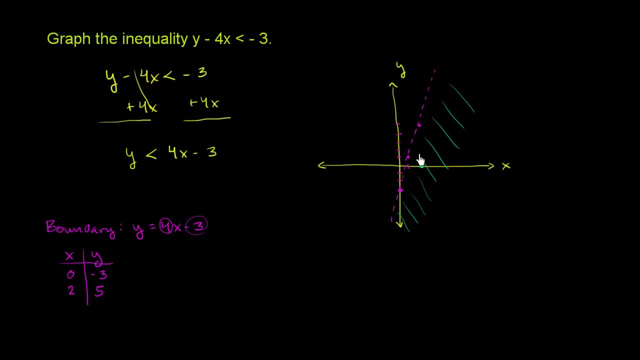 You can also try values out. You can say: well, this line is dividing our coordinate axes into, essentially, the region above it and the region below it, And you can test it out. Let's take something that's above it. Let's take the point 0, 0. 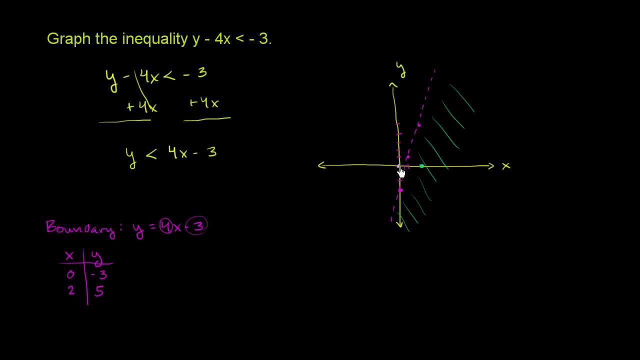 Let's take the point 0, 0 and see if that satisfies our inequality. If we have, y0 is less than 0 minus 3, or we'd get 0 is less than negative 3.. This is definitely not the case. 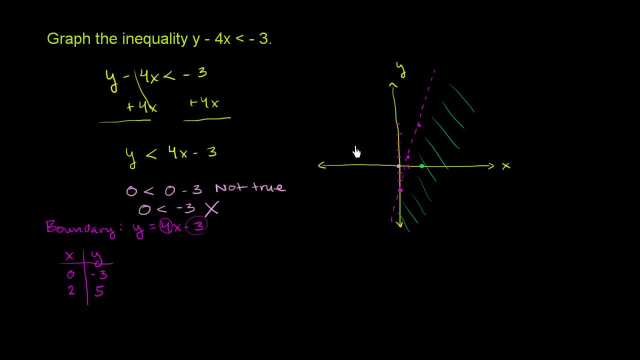 This is not true. This is not true And it makes sense, because that 0, 0 is not part of the solution. Now we could go on the other side, on the other side of our boundary line, And we could take the point. 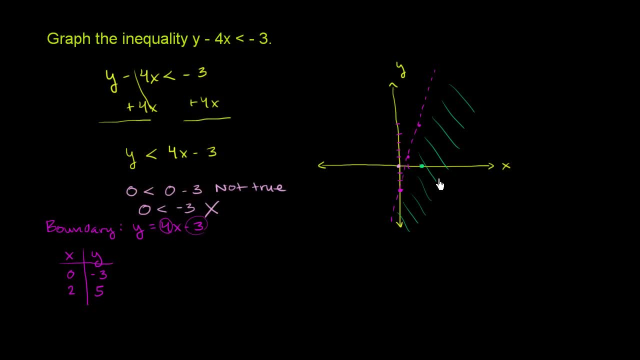 I don't know. Let's take the point 3, 0.. So let's say that this is the point. Well, that's right. There's the point 2, 0.. Let's take the point 3, 0 right over here. 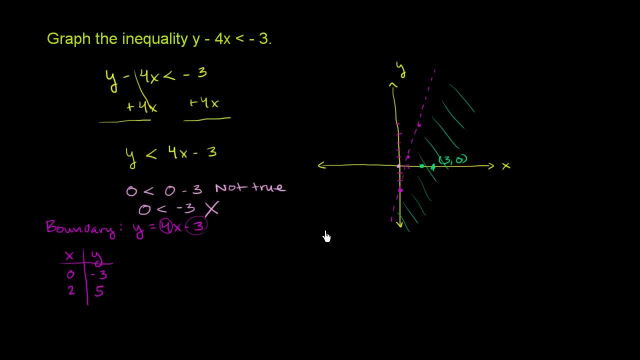 This should work because it's in the region less than. But let's verify it for ourselves. So we have: y is 0.. 0 is less than 4 times 3 minus 3.. 0 is less than 12 minus 3.. 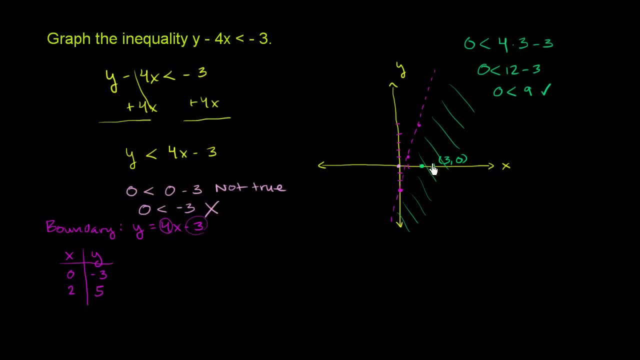 0 is less than 9, which is definitely true. So that point Does satisfy the inequality. So in general, you want to kind of look at this as an equal. to draw the boundary line, We did it, But we drew it as a dotted line because we don't want to include it. 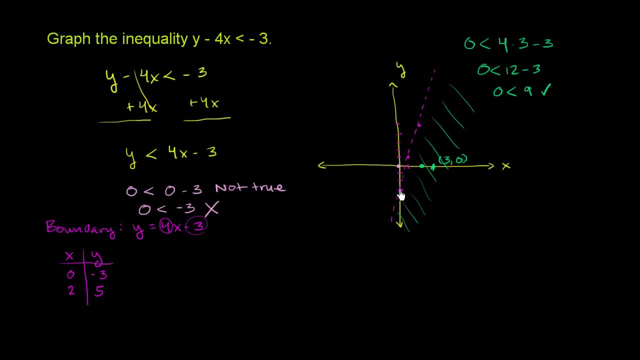 Because this isn't less than or equal to, It's just less than. And then our solution to the inequality will be the region below it, All the y's less than the line 4x minus 3.. 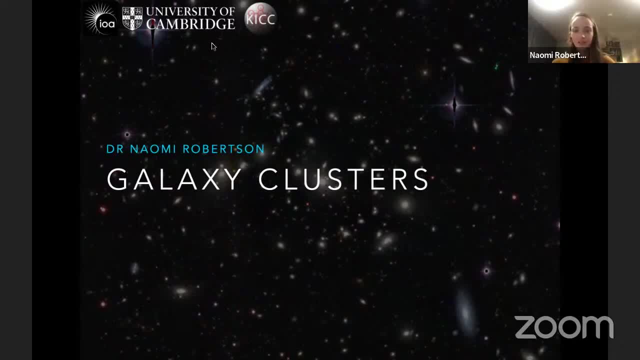 Hello everyone at home. welcome back to Wednesday evenings at Cambridge University Astronomy. It's a cloudy evening this week, so we have our headline speaker and then we're not going to stargating, but I think it's going to be a fascinating talk anyway. So we have Dr Naomi.